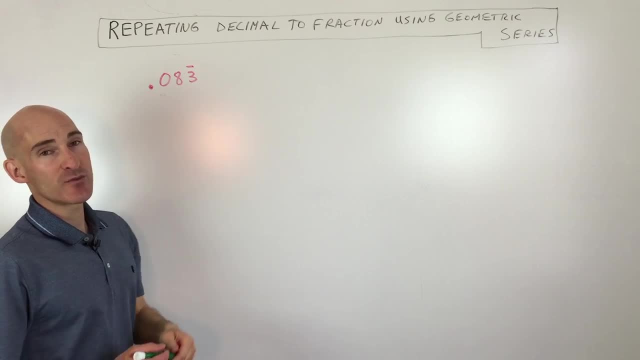 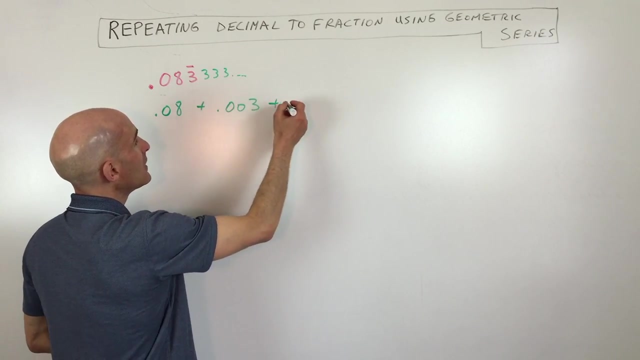 Point zero eight, three, repeating. and notice, it's just the three, that's repeating. and what students sometimes get confused by is: what do I do with the point zero eight? right, So what you want to do is you want to just separate out the point zero eight for a moment, So just write this as point zero eight. and what we're really interested in here is point zero zero, three, Okay, plus, because remember, this keeps going- three, three, three, Okay. this is the next term is going to be point zero, zero, zero, three, plus point zero zero three. 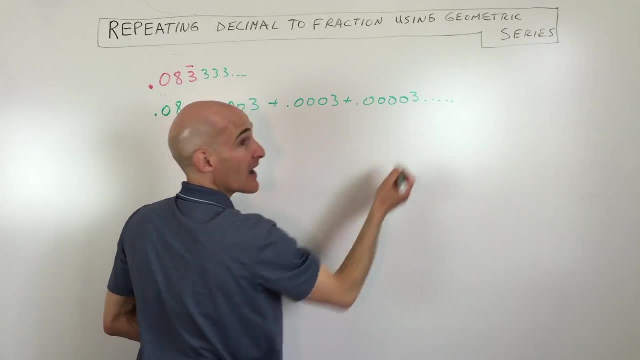 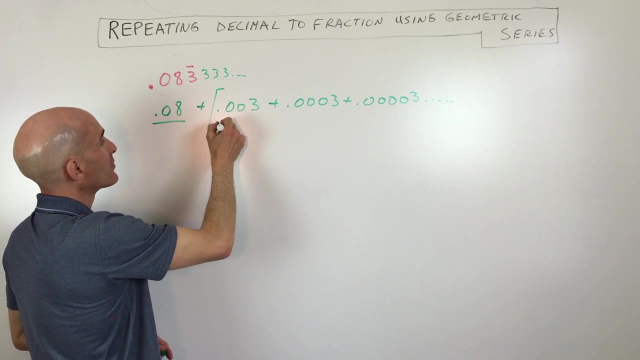 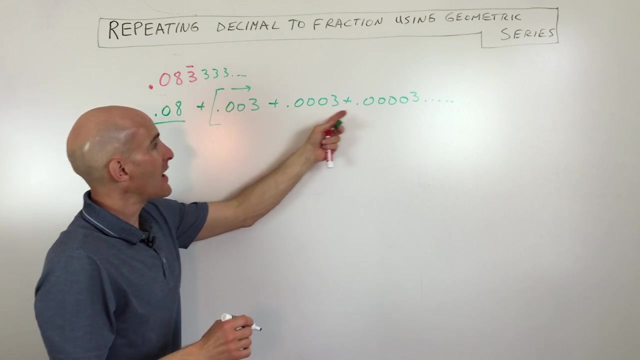 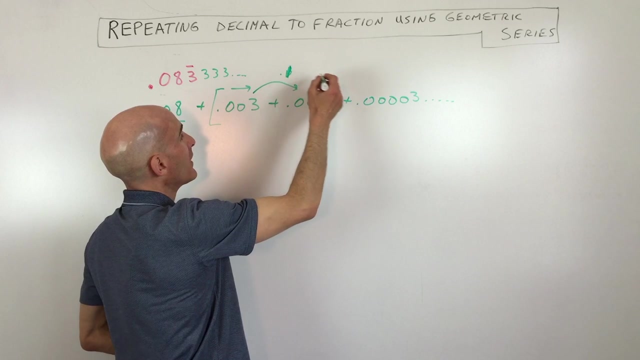 Point zero, zero, zero, zero, three, dot, dot, dot. Okay, so you can see this is a series, because we're adding the terms together. We're just going to ignore this point- oh eight, for a moment. We're just going to work with this part right here and then we'll add it in at the very end. So what you can see is that each time, what are we doing to get to the next term? Well, we're multiplying by point one. Okay, point one in the next term. Same thing, We're multiplying by point one. So whenever you move that decimal point, you know one to the left. 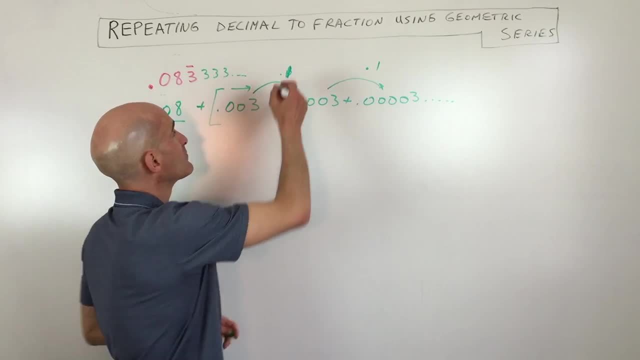 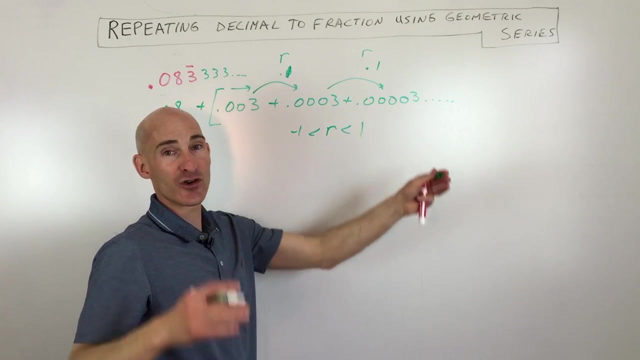 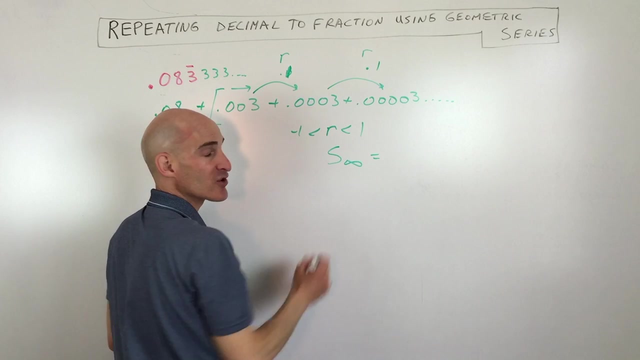 that's like dividing by ten, That's one tenth, which is point one, And this point one is the r value. That's the ratio, Okay, in a geometric series. So, since this is going on forever, Okay, it's an infinite geometric series. And since the ratio is in between negative one and one, Okay, we know, this is going to converge, It's going to get smaller and smaller, It's going to approach zero. We can add up all these terms using the infinite geometric series. Okay, the sum formula, Okay, which is a one over one minus r. Right. 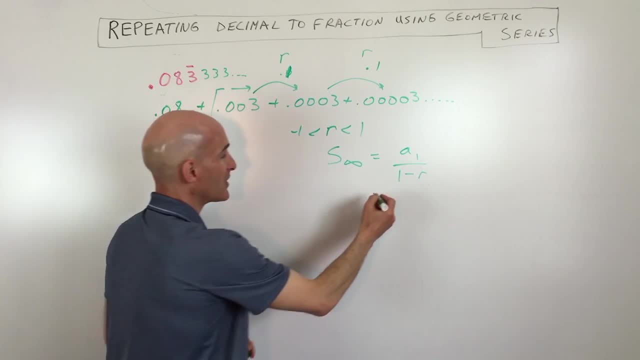 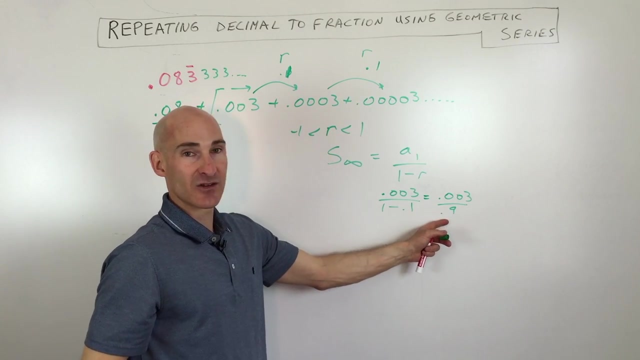 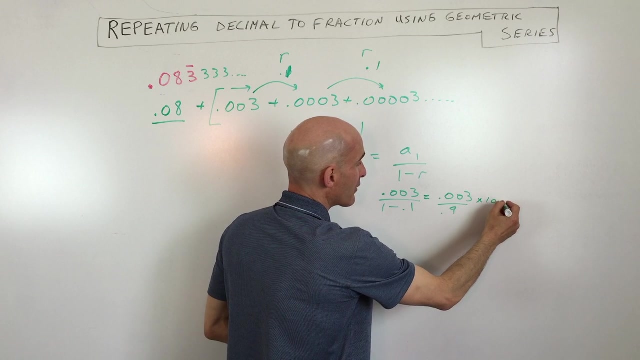 So the first term is point zero zero three. So point zero zero three over one minus point one. That's our ratio. So if we simplify this, we get point zero zero three over. Okay, point nine. Now you can see this is still decimals. here We want to convert this into a fraction, So let's see if we can get rid of these decimals. Let's multiply the top and bottom by 1000.. Okay, And so what that converts to is: it's going to be three.